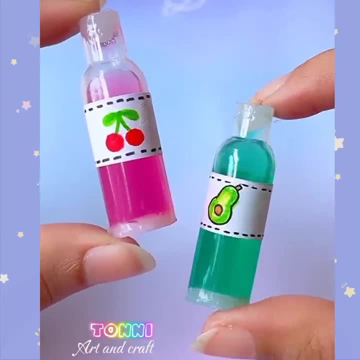 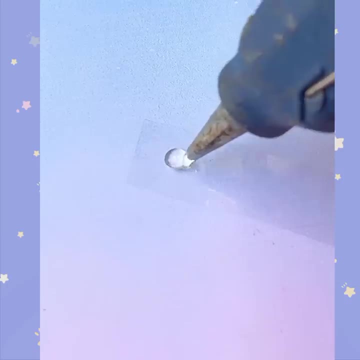 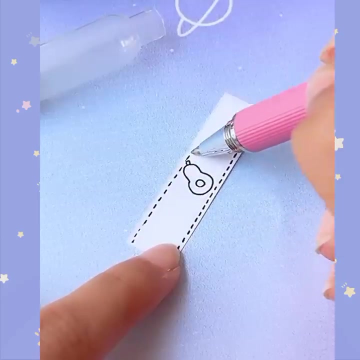 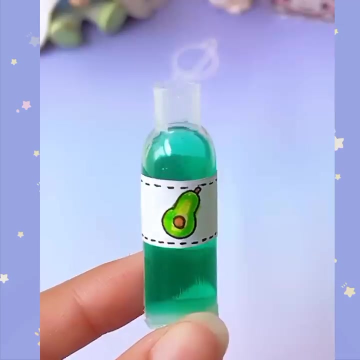 I'm thinking you were made for me. Isn't it my birthday yet? Cause I gotta say You're looking like a gift for me, Wrapped up, nice and neat. baby, Get in my way now, don't be shy, We'll be here dancing day and night. 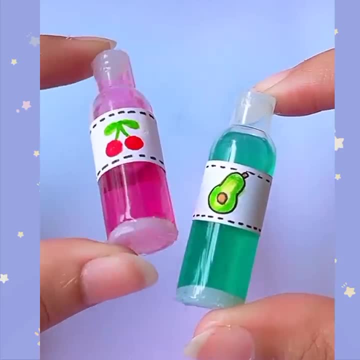 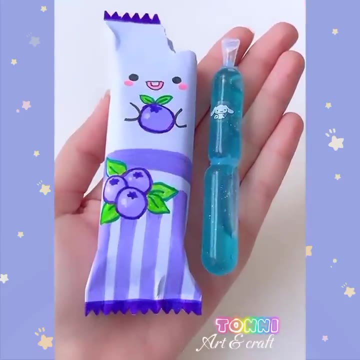 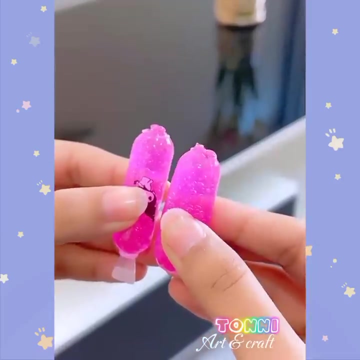 Get in my groove now. don't be shy, Cause I got this and some of my favorite things. You could be the part where it all begins. You could be the first and the second and the third and the rest of it. You could be one of the things I love. 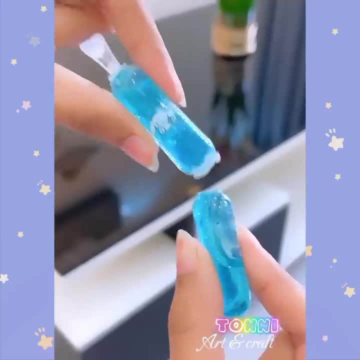 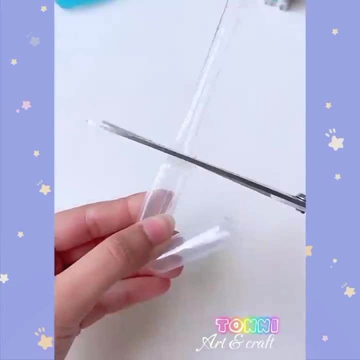 Sunday morning breakfast with a bedroom door locked. I like everything that has a jury on top. Get on my list of the things I love, love, love. You could be the one I trust, But those second chances, they are nothing for us. I like it when the jury on top. 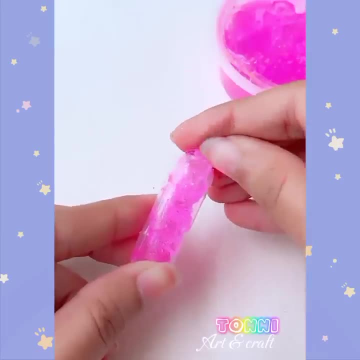 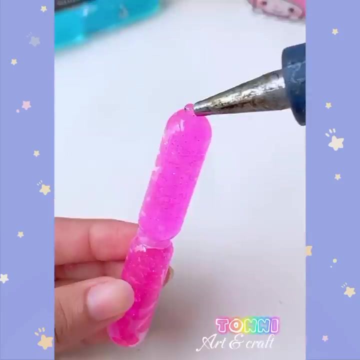 Be one of the things I love. We don't have to move so fast, Baby. I will show you how you can catch my vibe, And right away. I got so much time Looping in the blurry lights. Get in my way now. don't be shy. 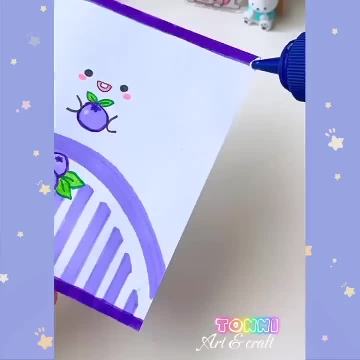 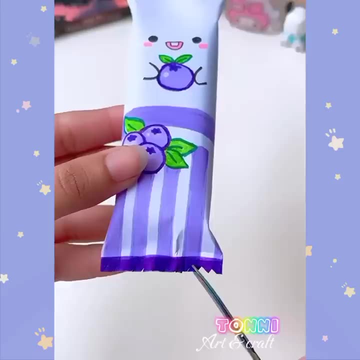 We'll be here dancing day and night. Get in my groove now, don't be shy, Cause I got this and some of my favorite things. You could be the part where it all begins. You could be the first and the second and the third and the rest of it. 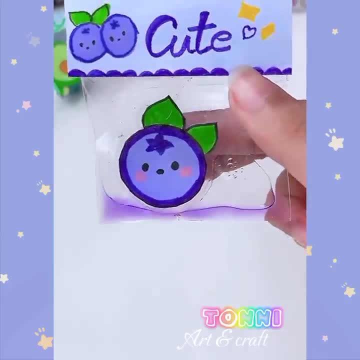 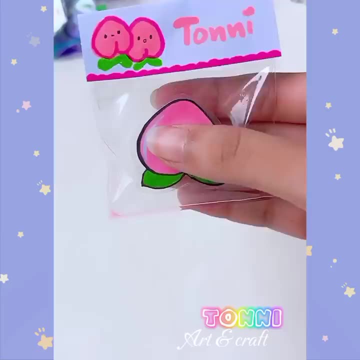 You could be one of the things I love: Sunday morning breakfast with a bedroom door locked. I like everything that has a jury on top. Get on my list of the things I love, love, love. You could be the one I trust. But those second chances, they are nothing for us. 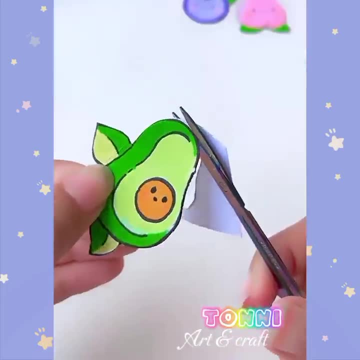 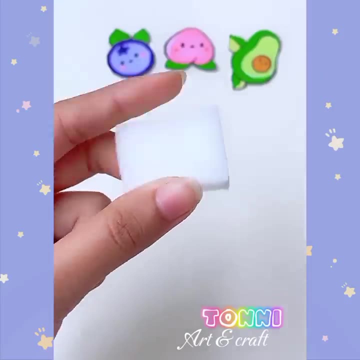 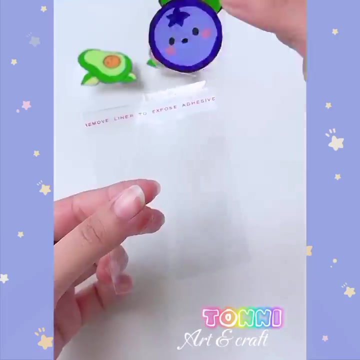 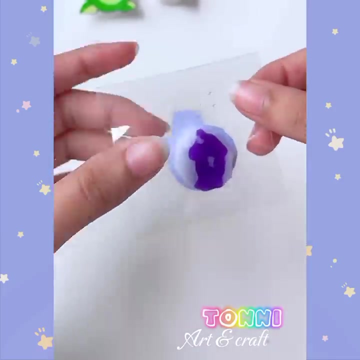 I like it when the jury on top: Be one of the things I love, The things I love, love, love and the rest of it, The things I love, love-love-love, love, love-love, Out of the things I love. Be one of the things I love, The things I love, love-love-love. 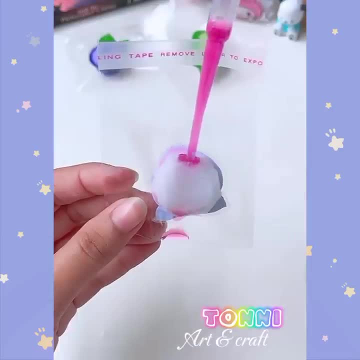 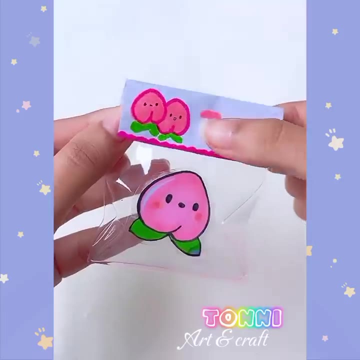 Cuz. I think it's still my favorite thing. This, too, could be the part where it all begins. We could be the first, and the second, and the third and the rest of it. Get in my way now. don't be shy. We'll be here dancing day and night. 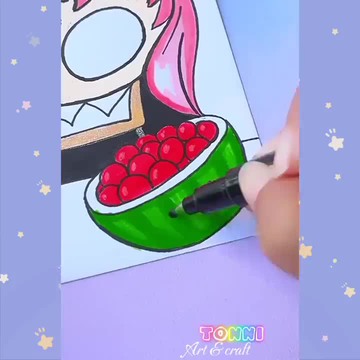 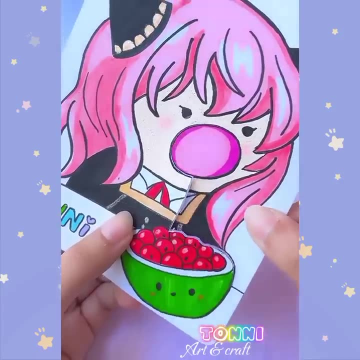 Get in my groove now. don't be shy. You could be one of the things I love: Sunday morning breakfast with our bedroom door locked. I like every tingling. that's a cherry on top. Get on my list of the things I love, love, love. 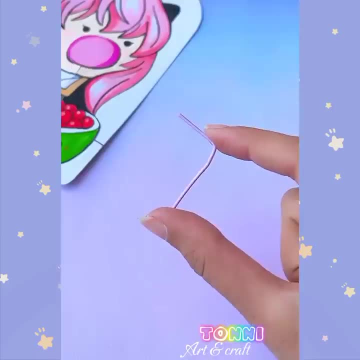 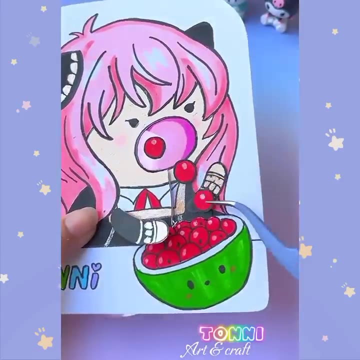 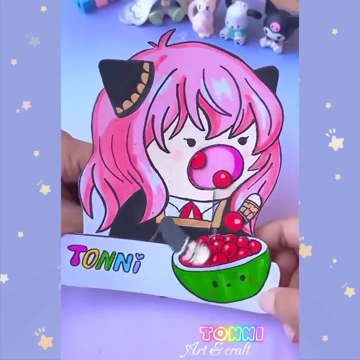 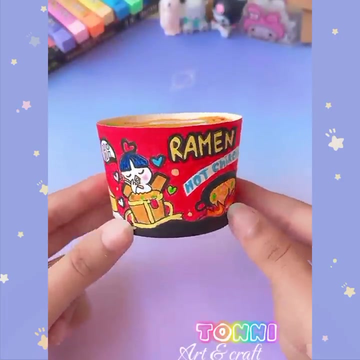 You could be the one I trust All those second chances. they are nothing for us. I like it all with the cherry on top. Be one of the things I love, The things I love, the things I love. Be one of the things I love. I've heard of any rising. 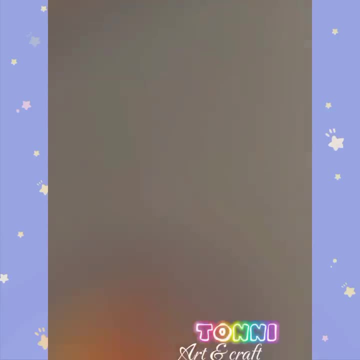 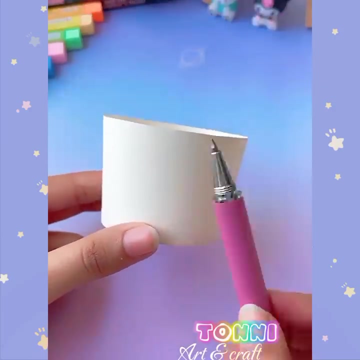 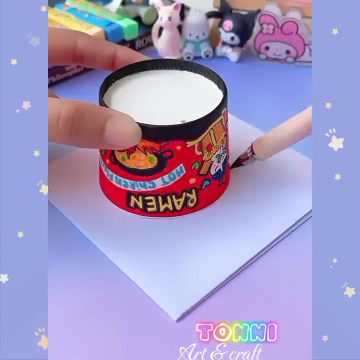 The color among you see brightest lightning. I've heard of any rising Already memories. Now, I just don't really care What you feel. what you feel, what you feel. Show you about me Thinking it was just a phase. Got me like ooh, got me like ooh. 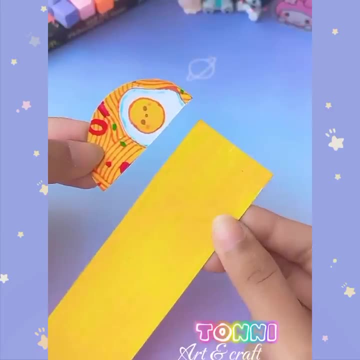 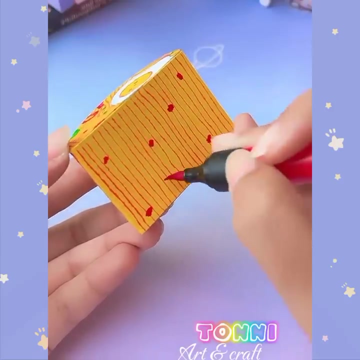 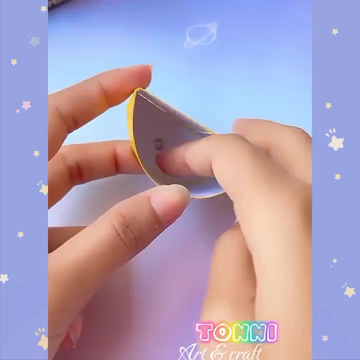 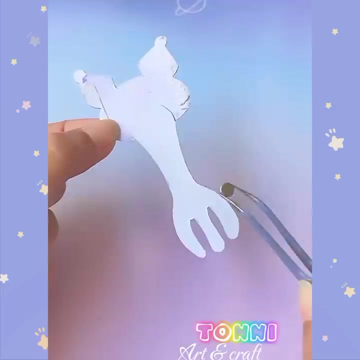 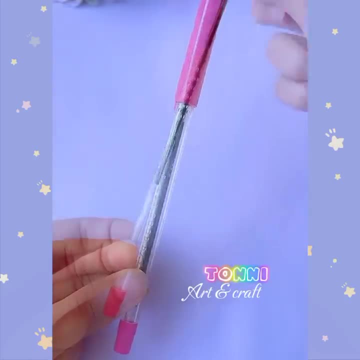 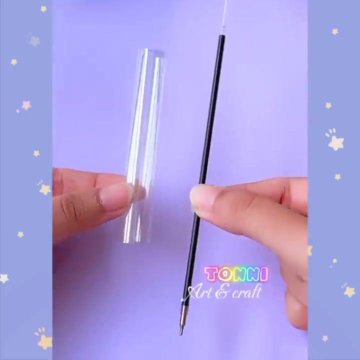 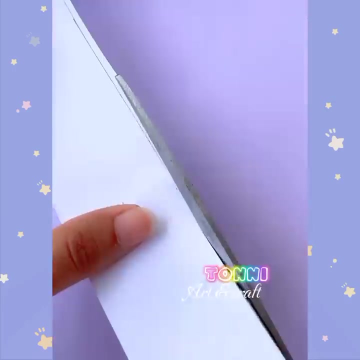 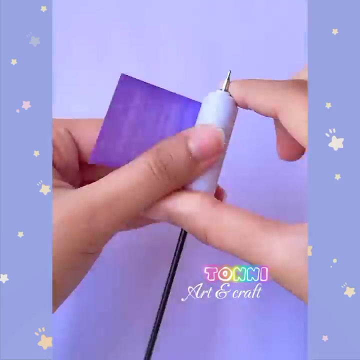 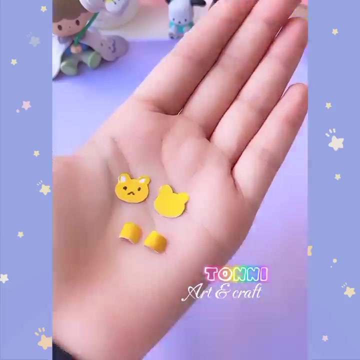 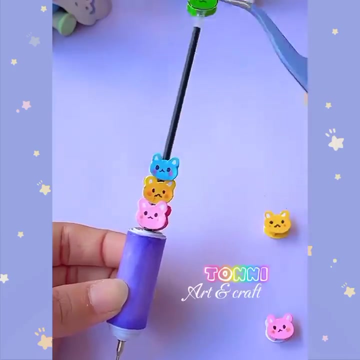 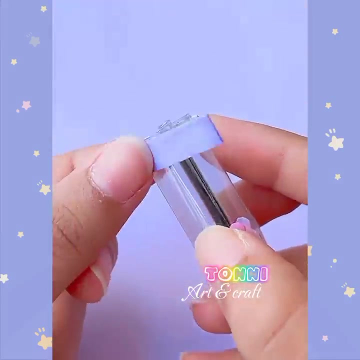 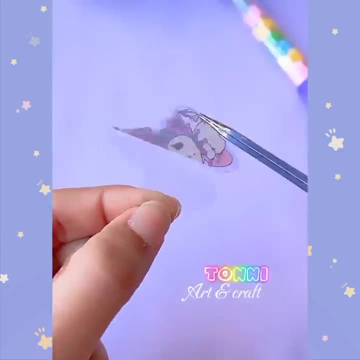 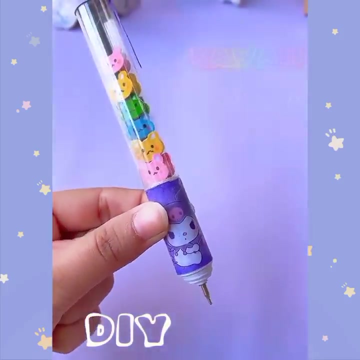 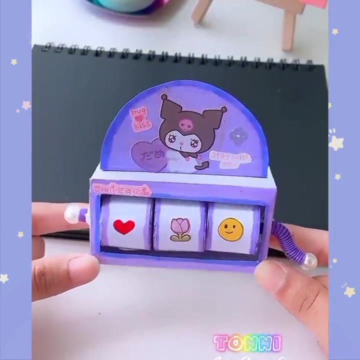 shower of love right there. what? how you think? Shame on me thinking it was just a fake. Got me like ooh. got me like ooh. Ain't no fun recognizing your mistake. Got me like ooh, feelings like ooh. Now I brought my worst behavior. 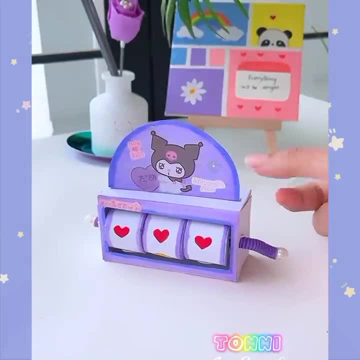 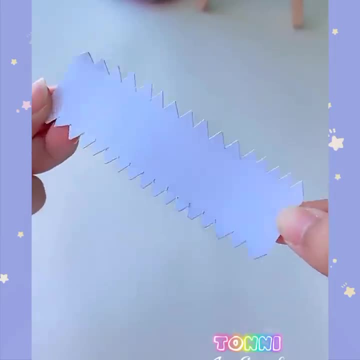 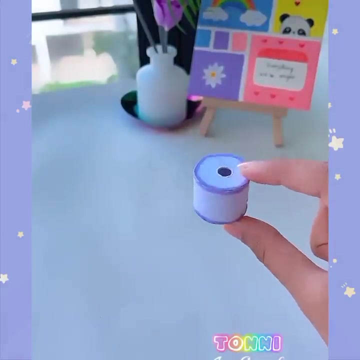 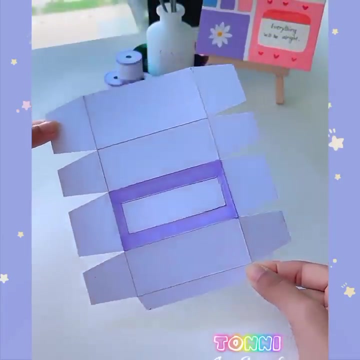 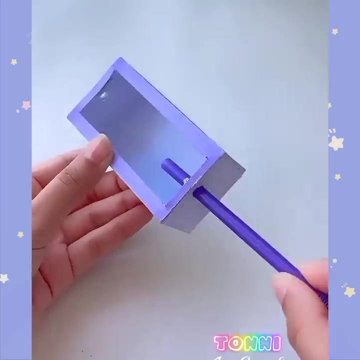 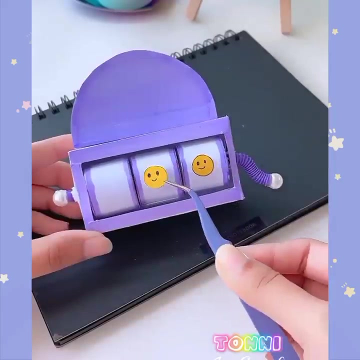 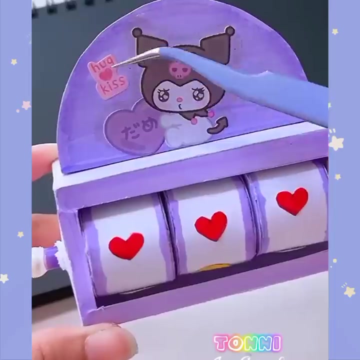 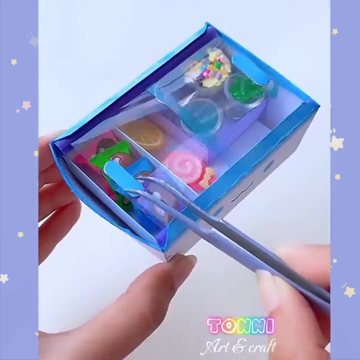 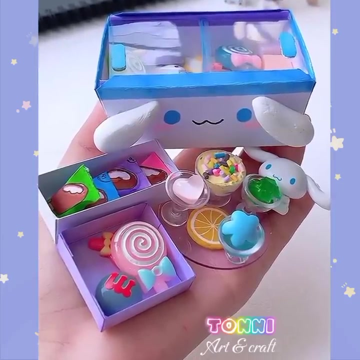 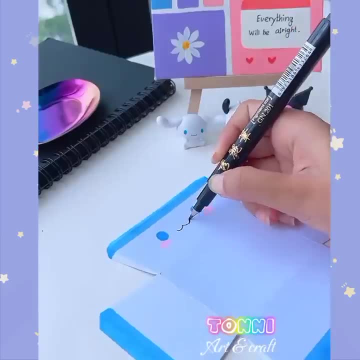 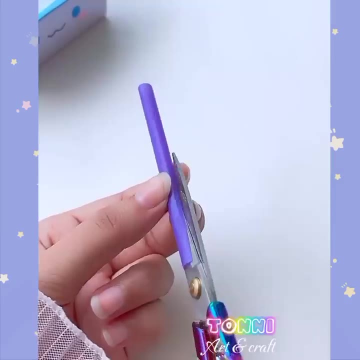 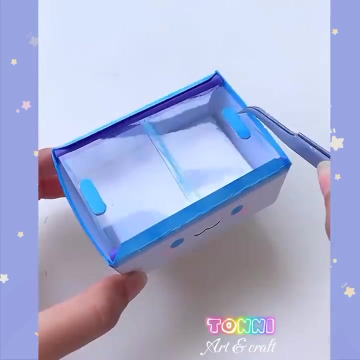 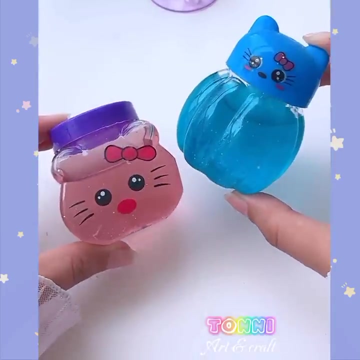 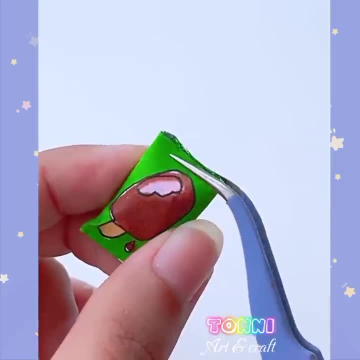 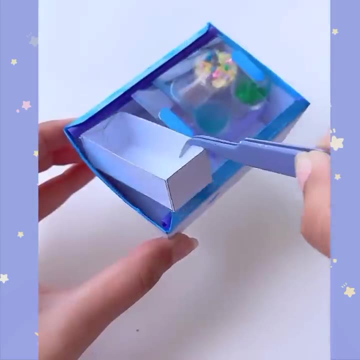 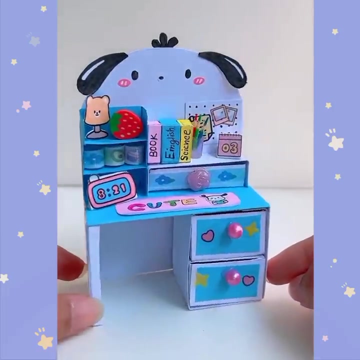 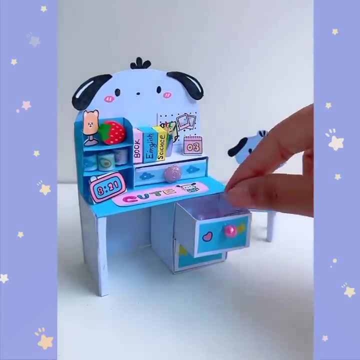 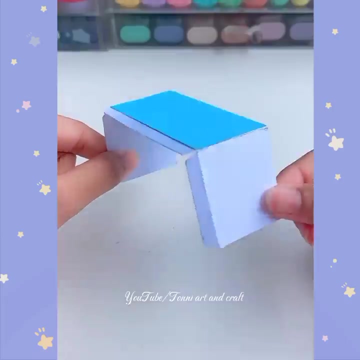 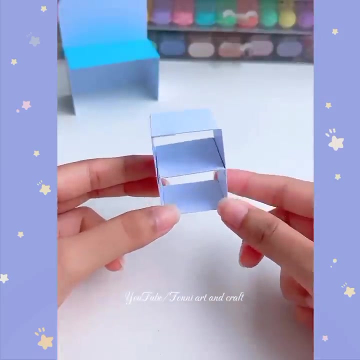 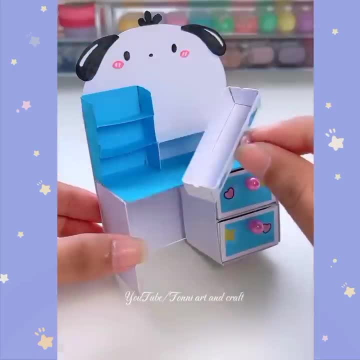 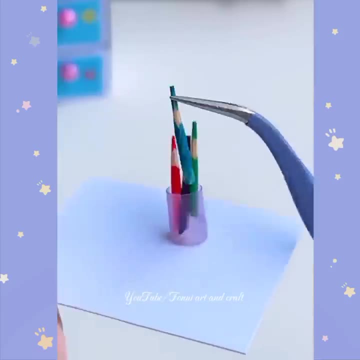 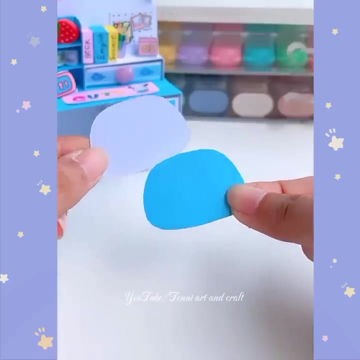 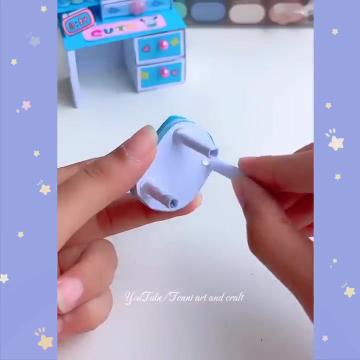 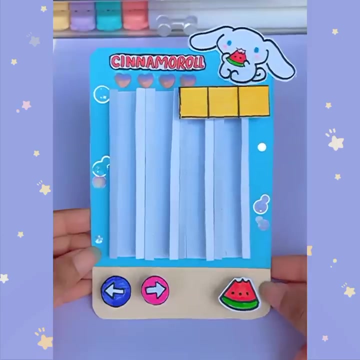 I just wanna flow like a ship Made out of paper. Right now I need to Take care of myself, Comforting myself Like a rollercoaster. One week I'm up, Next one I'll be down. But I'm getting closer to A stronger me Feeling free Like a rollercoaster. 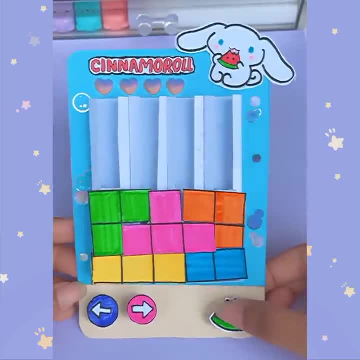 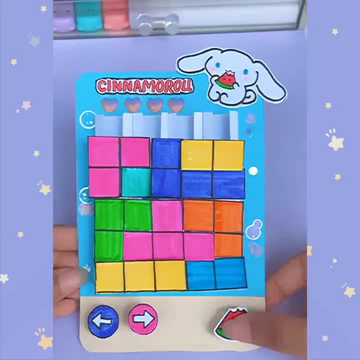 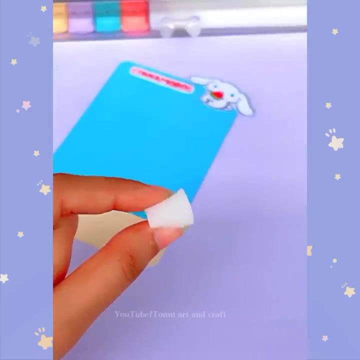 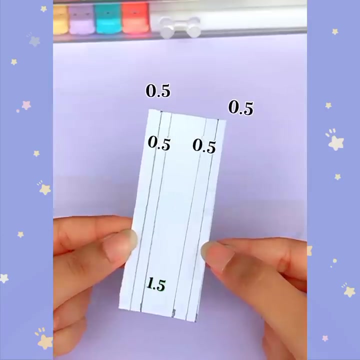 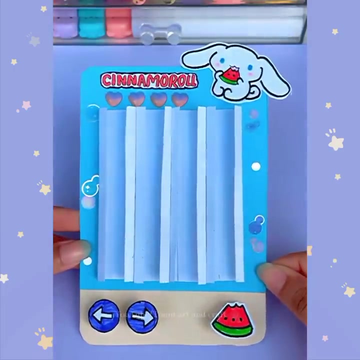 A stronger me Feeling free Like a rollercoaster. Grandpa used to ask Why I'm single with such a pretty face. Where is your man? You should go out and chase him Now. I'm so tired of breathing underwater, I just wanna flow like a ship. 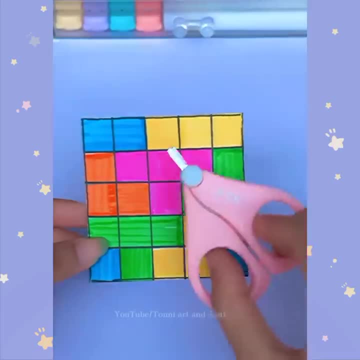 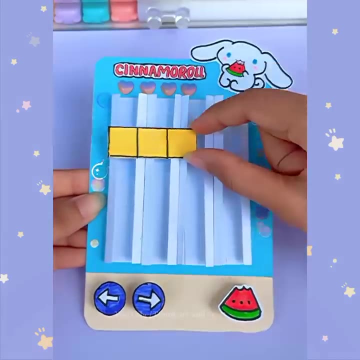 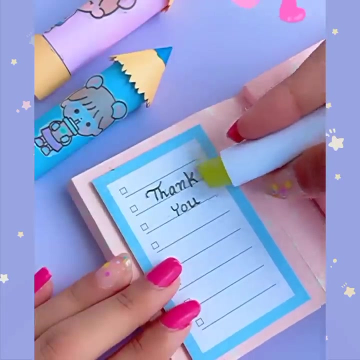 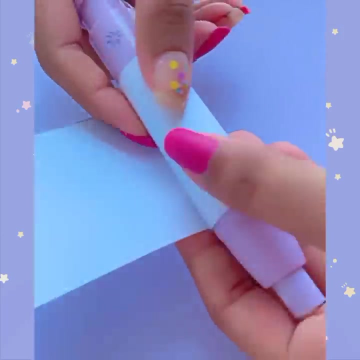 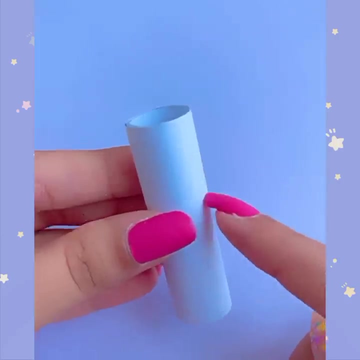 Made out of paper. So now I'm about to Take care of myself, Comforting myself Like a rollercoaster: One week I'm up, Next one I'll be down. But I'm getting closer to A stronger me, Feeling free Like a rollercoaster- Stronger me. 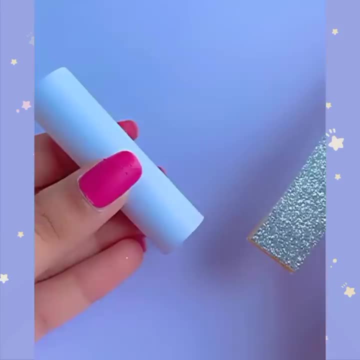 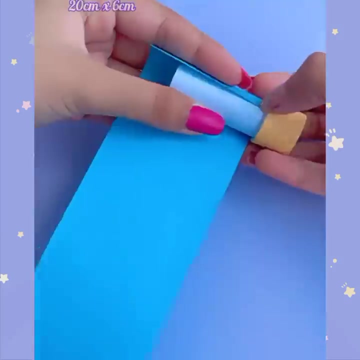 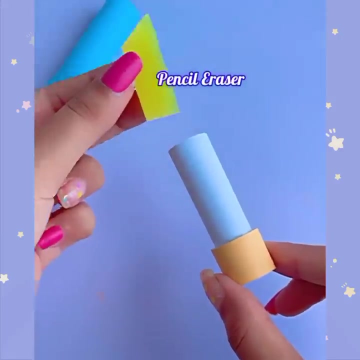 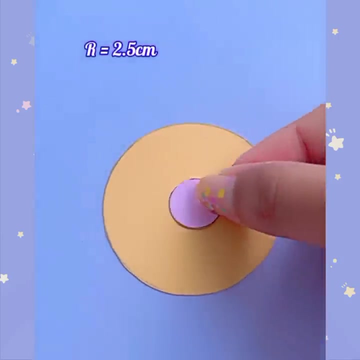 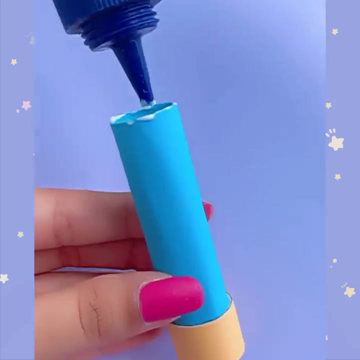 Feeling free Like a rollercoaster. I don't need anyone else, I just wanna be for myself A while. nobody else, I just need myself, Take care of myself, Comforting myself Like a rollercoaster. One week, I'm up, Next one, I'm up. One week, I'm up. 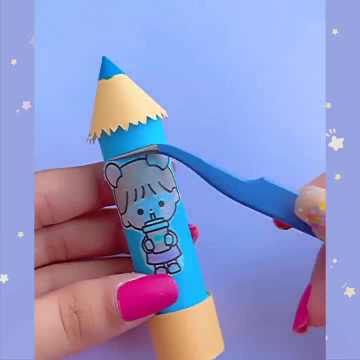 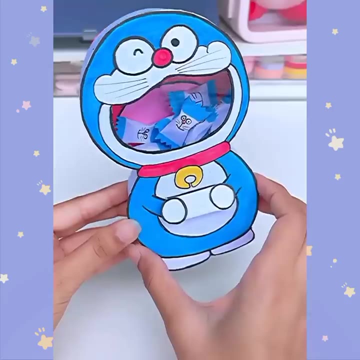 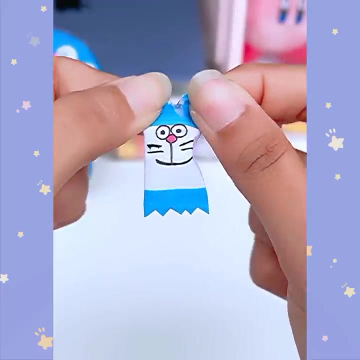 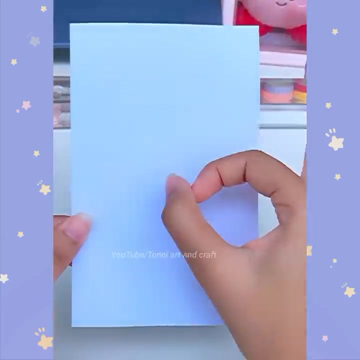 Next one I'll be down, But I'm getting closer to A stronger me Feeling free Like a rollercoaster. Stronger me Feeling free Like a rollercoaster. Always my own damn fault that I fall and break. It's my fault that I fall and break.